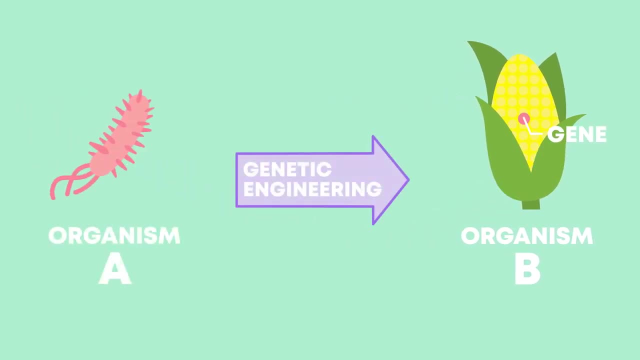 from a different organism introduced to give it some advantage that has naturally. Organisms like are called genetically modified or transgenic organisms. For example, a gene that manufactures a toxic chemical in a bacterium can be introduced into a maize plant to make the plant toxic to certain insects that would eat it, such as caterpillars. 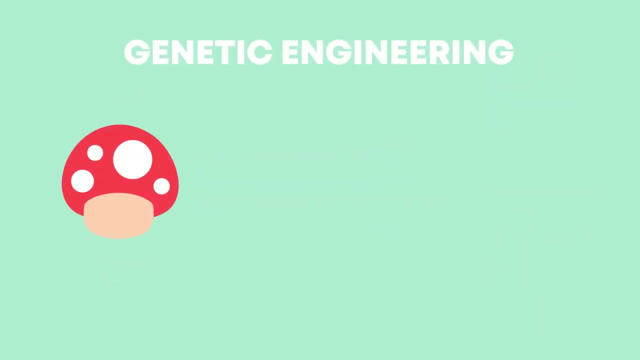 Let's now look at the process of genetic engineering. How do you transfer a genetic characteristic from one organism to another? Although it's a very complex process, it can be summarized rather simply. We'll use the example of how the insulin gene is inserted into a bacterium. 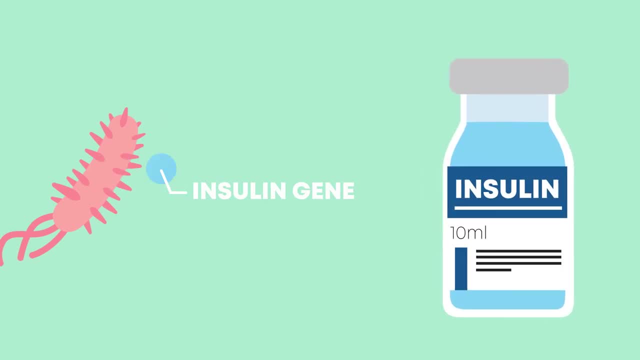 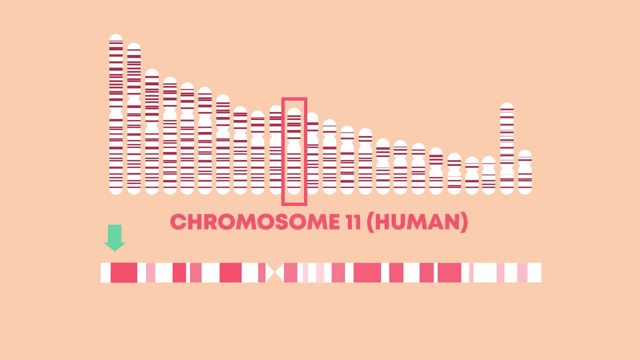 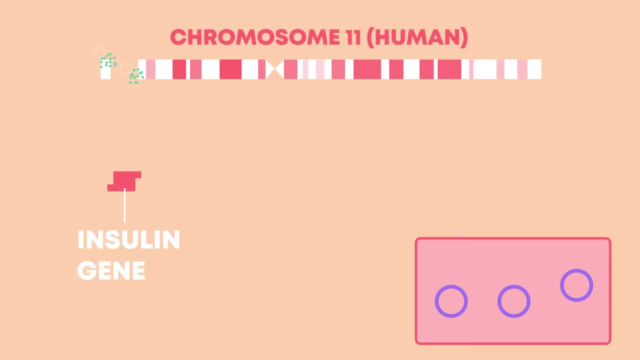 in order to manufacture large amounts of bacteria. The gene that codes for human insulin is found on chromosome 11 at position 15.5.. The insulin gene is cut from chromosome 11 using special enzymes called restriction enzymes. Bacteria possesses small circular strands of DNA floating in their cytoplasm. These 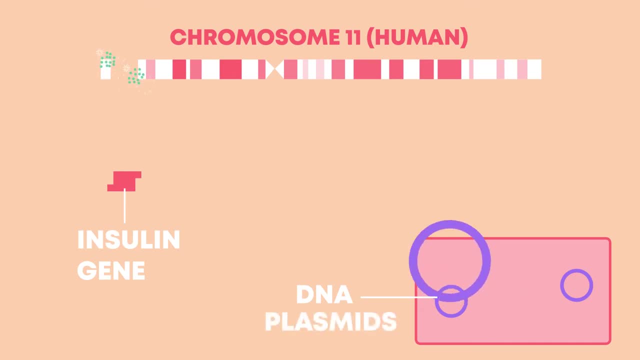 strands of DNA are called plasmids. A plasmid is extracted from the bacterium cell. The plasmid is cut open using the same restriction enzymes that were used to cut the insulin gene from the human chromosome. The restriction enzymes leave sticky ends where one of the two DNA 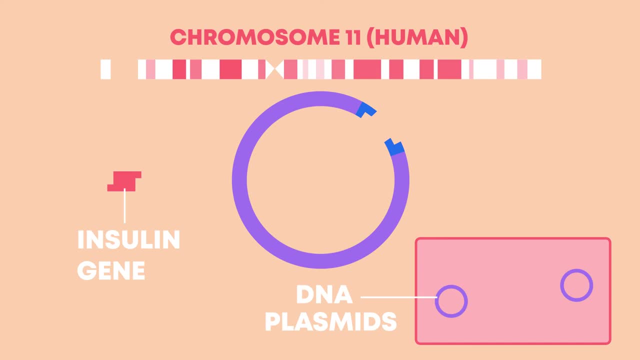 strands is slightly longer than the other Because the same restriction enzyme was used to cut both the human DNA and the bacterial plasmid. the sticky ends are complementary and will allow for joining using complementary base pairing. The insulin gene is joined to the plasmid by the 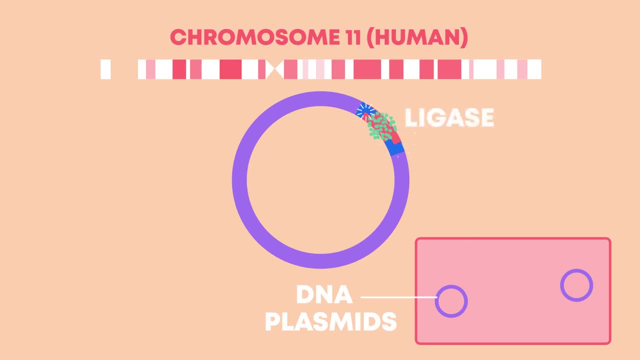 sticky ends, An enzyme called ligase is used to complete the joining of the two pieces of DNA. The modified plasmid is then reinserted into the bacterial cell. The modified bacterium is a genetically modified or transgenic organism, because it contains some human DNA, along with 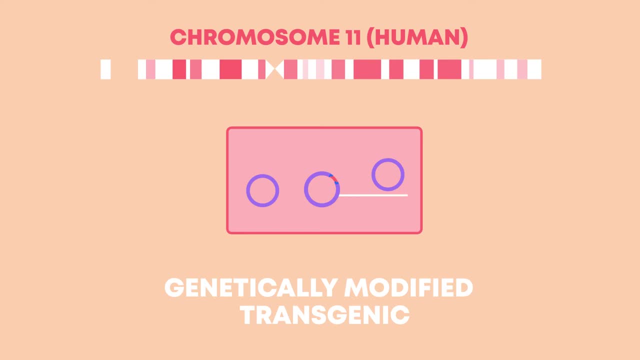 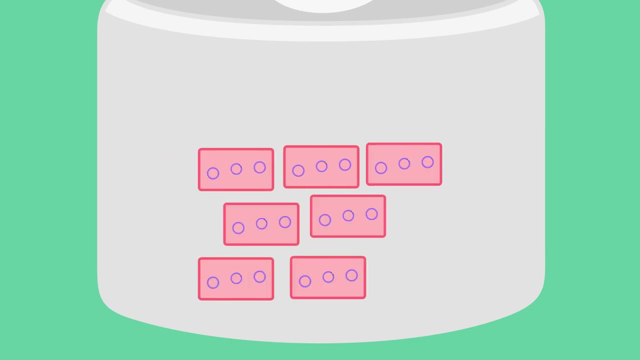 its own bacterial DNA. Its bacterial DNA is called recombinant DNA, bacterial DNA recombined with human DNA. The bacterial cell is placed in a fermenter which allows for rapid asexual reproduction in ideal conditions, with the optimal temperature, pH and lots of food Because the bacteria reproduce.